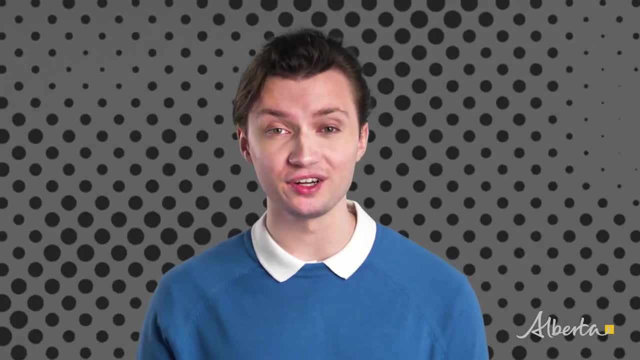 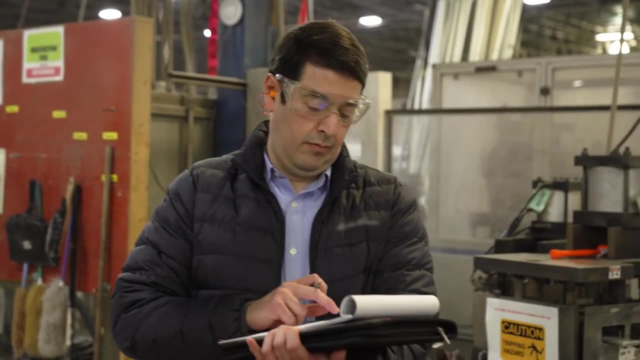 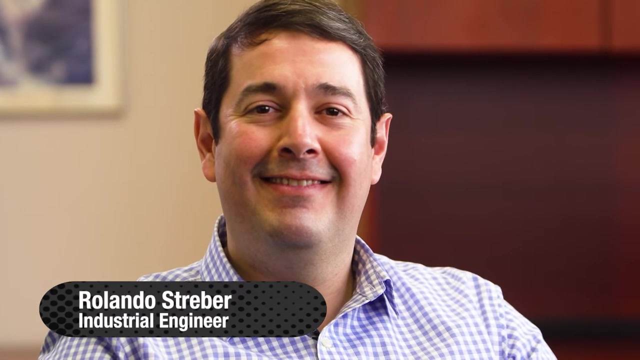 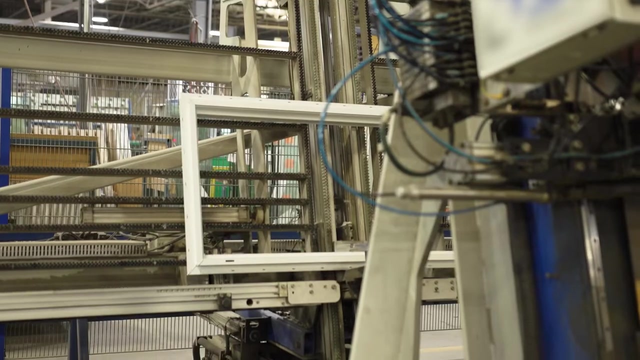 To help us process the details of this career, we talked to an industrial engineer working here in Alberta. Hi, my name is Rolando and I'm an industrial engineer. An industrial engineer typically designs, develops, improves and implements systems comprised of materials, people, equipment and energy. 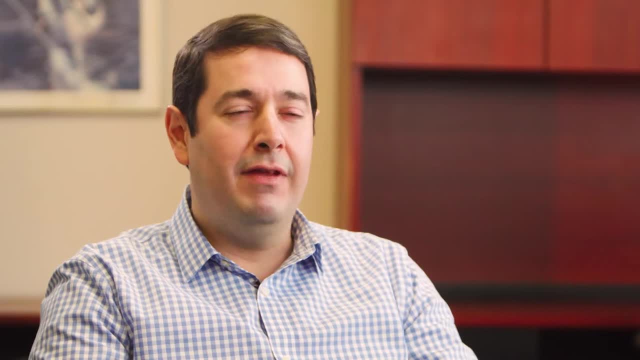 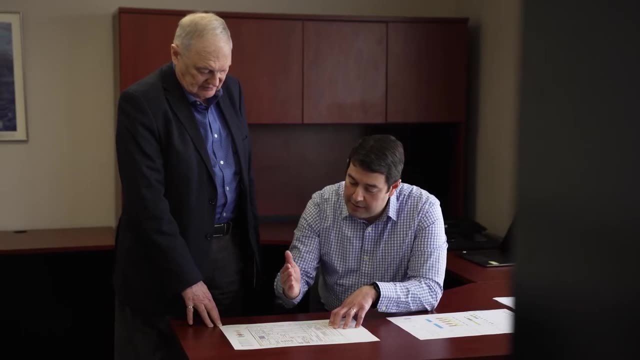 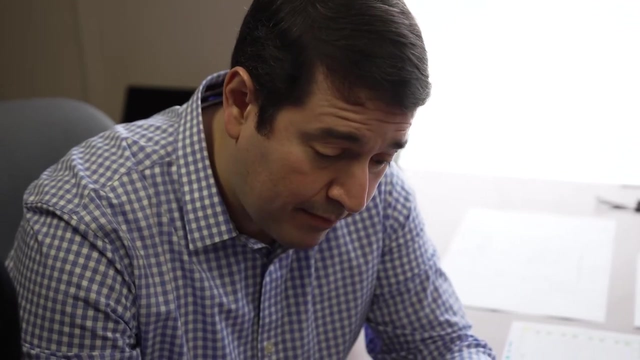 And our work typically helps to improve productivity, quality and efficiency. As an industrial engineer, you can work in any industry as long as there is a process for you to analyze and improve. So you can find yourself working in the finance sector, healthcare, manufacturing, supply chain and logistics, to name a few. 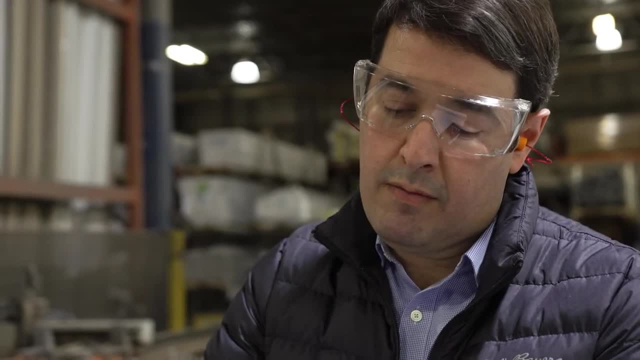 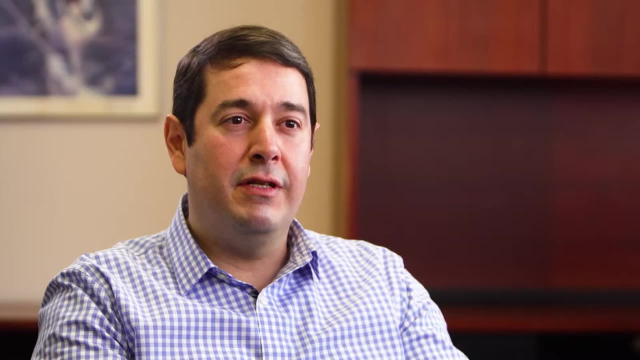 I enjoy being an industrial engineer because you can affect in a positive way people's life by making their workplace better, and also because you can help organizations to improve their systems and processes. A typical day for me depends on what project I'm working on. 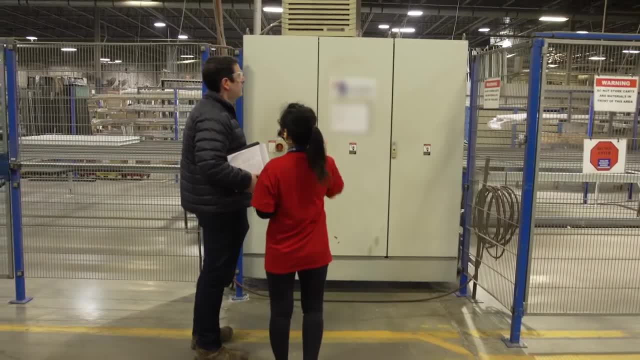 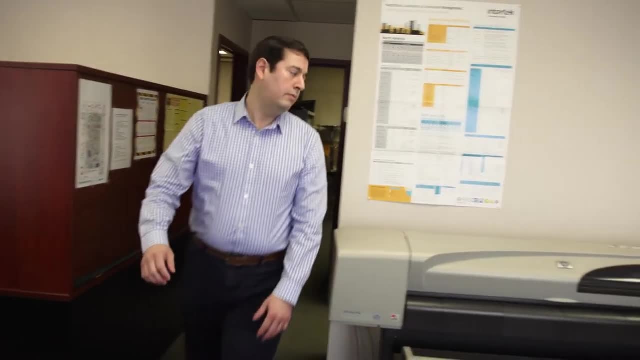 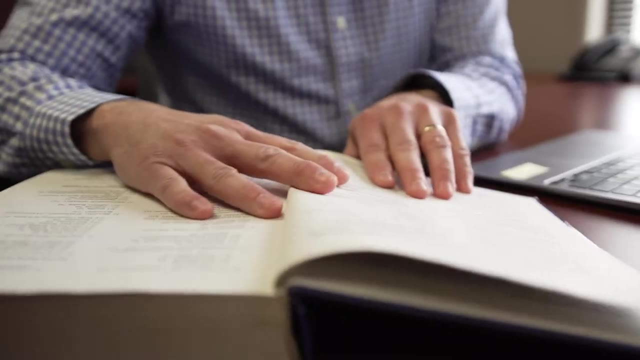 I can find myself working in a site as a manufacturing facility or a warehouse, collecting information or making observations. I'll come back into my office and process all that data. Then I'll use that data, analyze it and get a solution for the problems that we are studying. 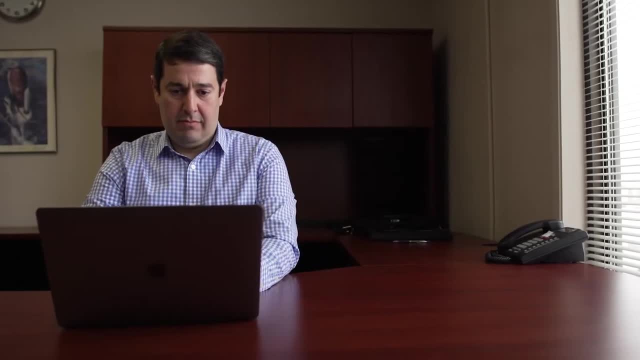 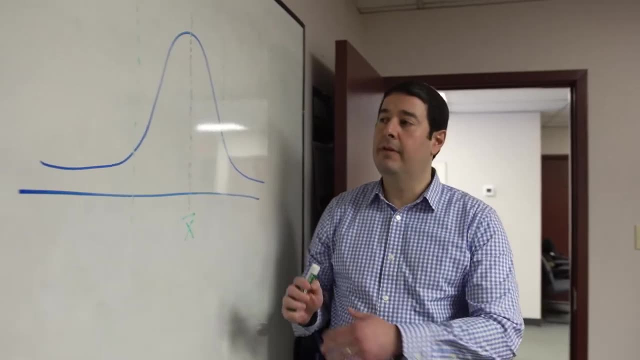 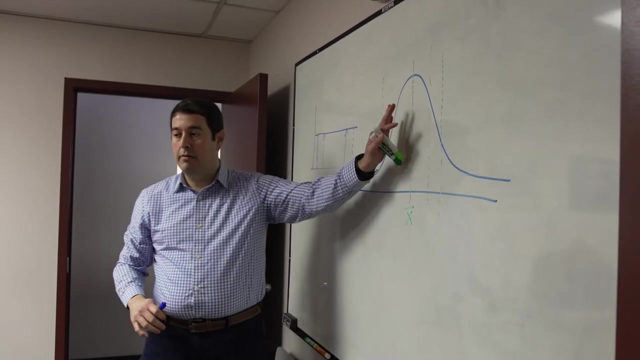 After that I can find myself creating a report. We also have multiple meetings with stakeholders or with clients. Sometimes I'll find myself presenting those reports to our clients. As an industrial engineer, your duties vary depending on the project you're working on at the time. 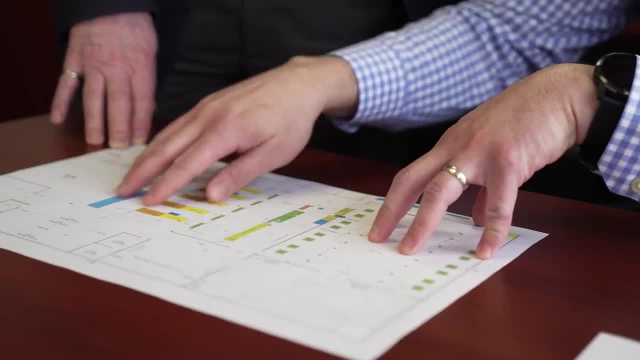 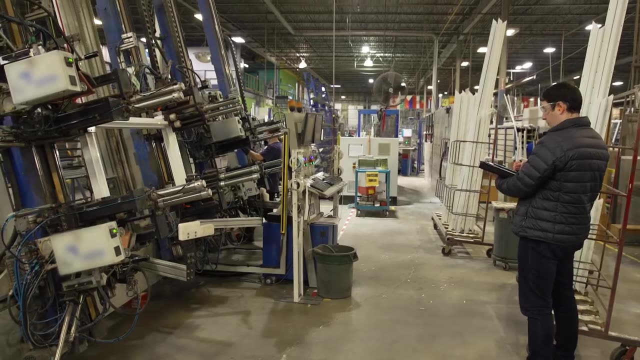 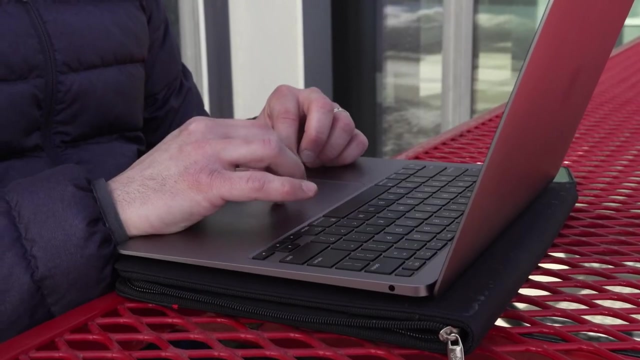 but some of them include defining the problem. what is it you're going to study, planning the execution of the project and collecting the data and analyzing all that information To solve the problem. you use many different types of software to build simulation models. 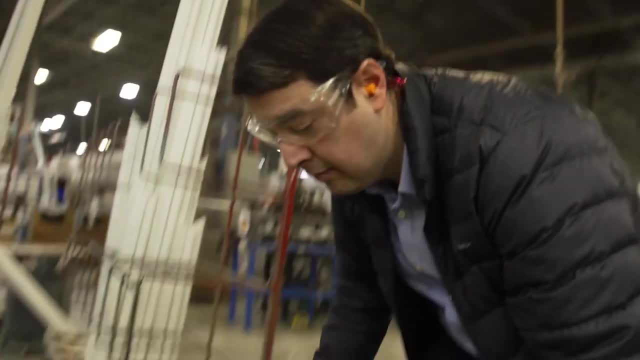 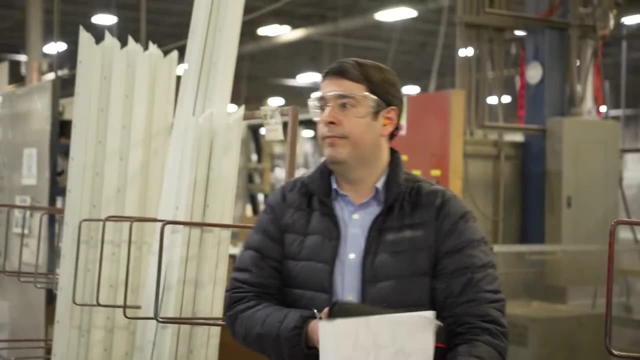 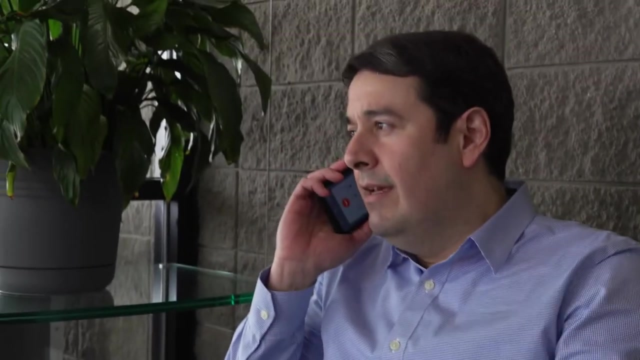 As an industrial engineer, you've got to have people skills, math. you will need communication skills and the ability to visualize the effects of change. It is also very important to have an interest in people and systems. As an industrial engineer, you have many deadlines.